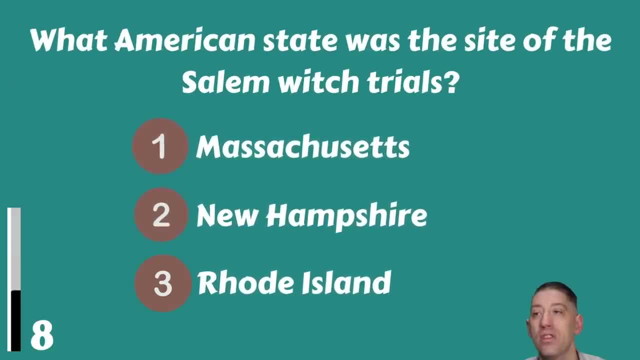 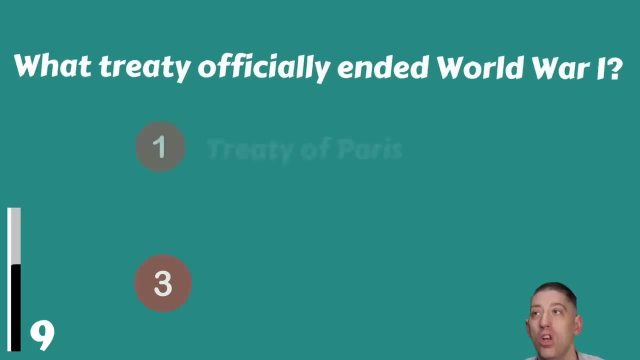 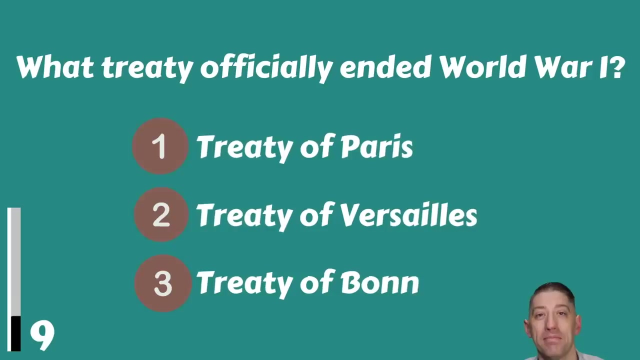 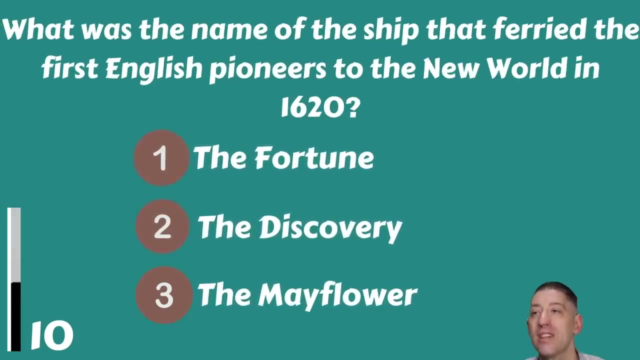 what american state was the site of salem witch trials? massachusetts, new hampshire or rhode island, massachusetts? what treaty officially ended world war one? the treaty of paris, the treaty of versailles or the treaty of bonn? the treaty of versailles? what was the name of the ship that ferried the first english pioneers to the new world in 1620? 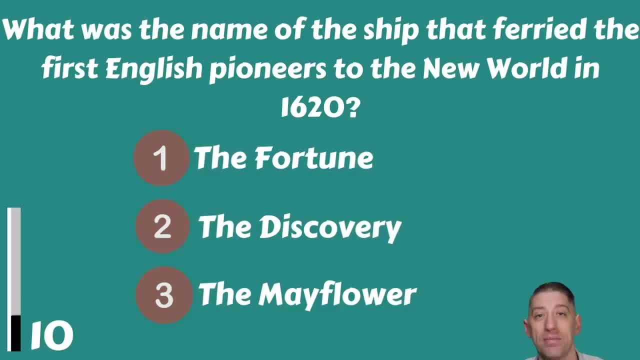 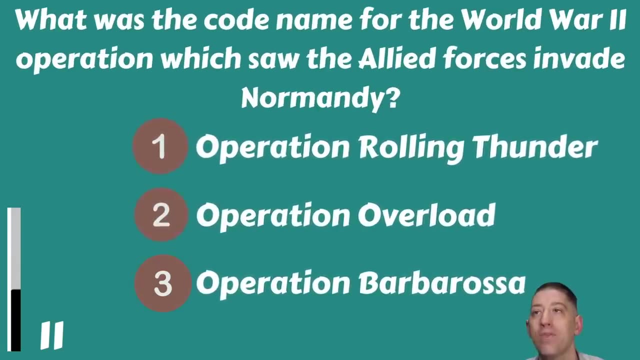 the fortune, the discovery or the mayflower? what was the name of the ship that ferried the first english pioneers to the new world in 1620? the fortune, the discovery, or the treaty of paris, the treaty of versailles or the treaty of bonn, the沒錯? 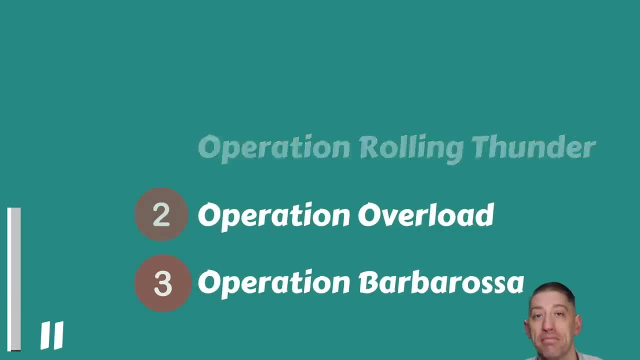 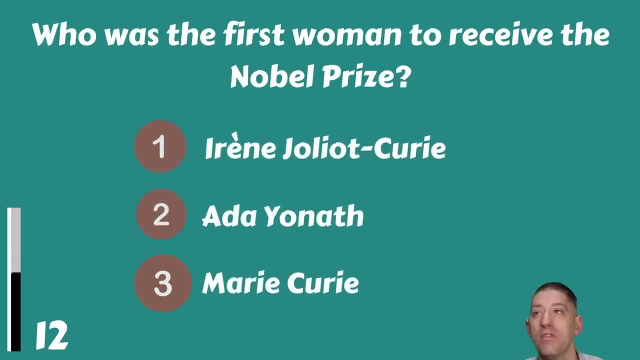 what was the code name for the world war ii operation which saw the allied forces invade normandy? operation rolling thunder, operation overlord or operation barbarossa? woman to receive the Nobel Prize? Irene Joliet-Curie, Ada Yonath or Marie Curie? 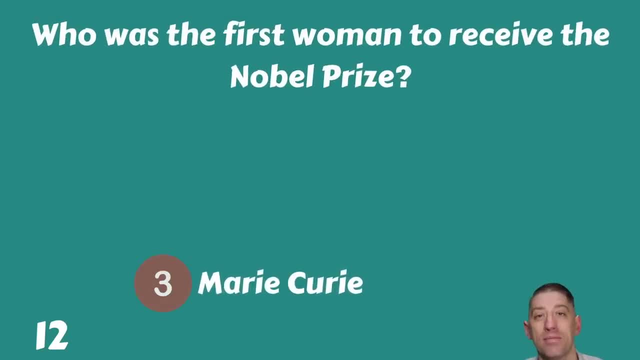 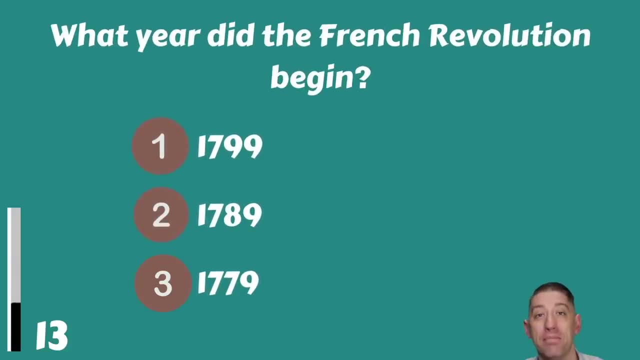 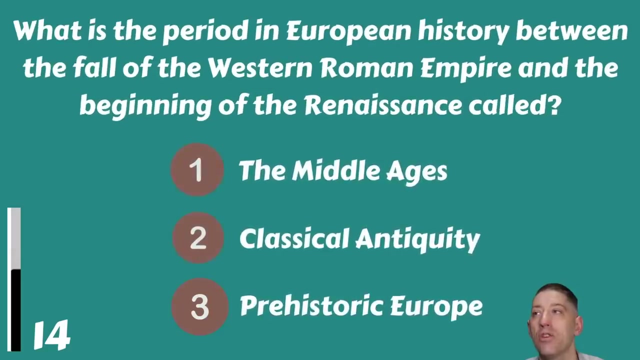 Marie Curie. What year did the French Revolution begin? 1799,, 1789, or 1779? 1789,, 1789, or 1789?? What is the period in European history between the fall of the Western Roman Empire and the? 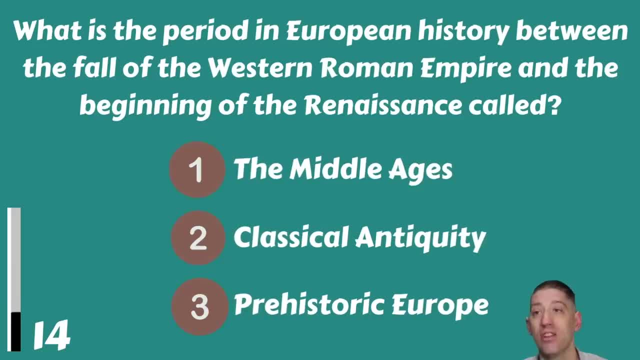 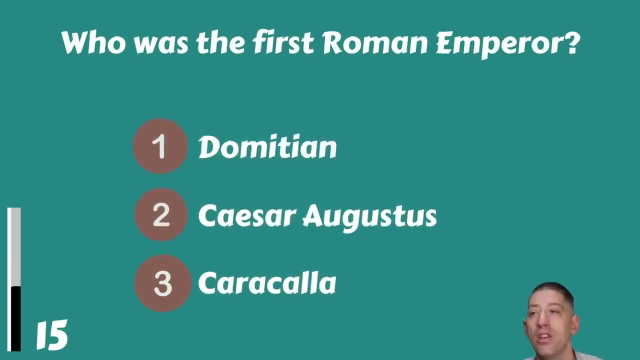 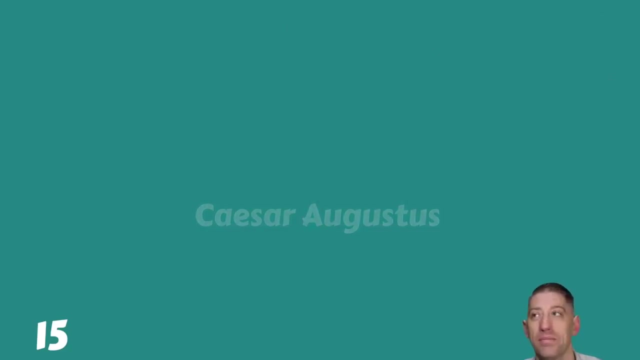 beginning of the Renaissance, called The Middle Ages, Classical Antiquity or Prehistoric Europe, The Middle Ages. Who was the first Roman emperor to be born? Caesar Augustus or Caracalla Caesar Augustus? Which architect is famous for the dome of Florence Cathedral in Italy? 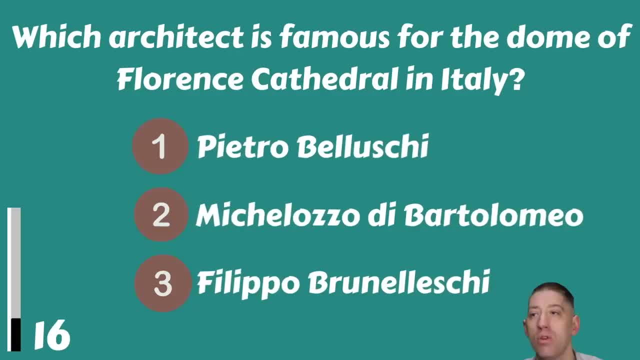 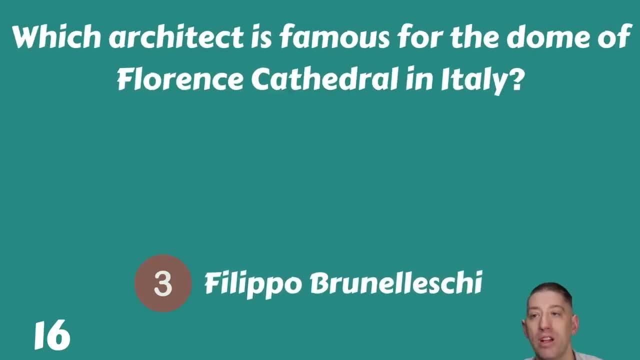 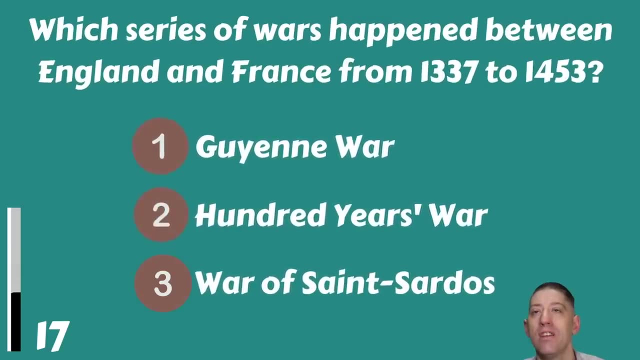 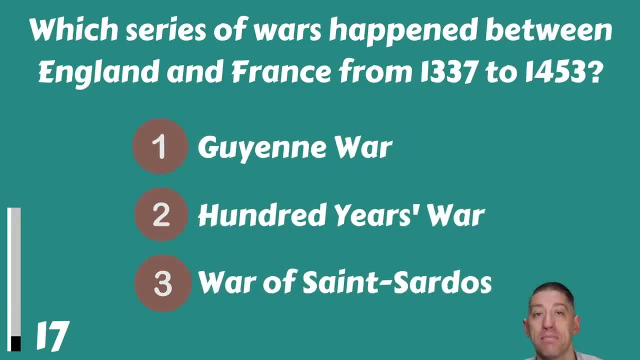 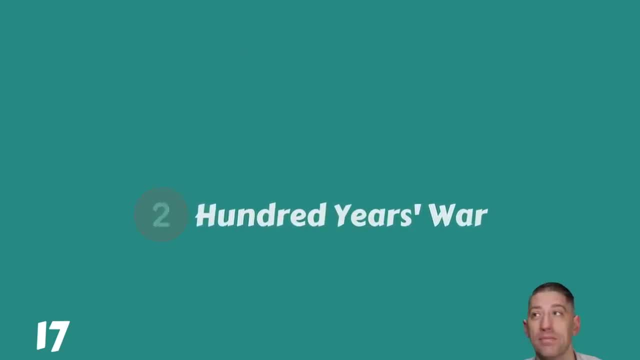 The Goyenne War, the Hundred Years' War, or the War of St Sardos, The Hundred Years' War? Who is credited with the creation of the first practical light bulb? James Watt, Nikola Tesla or Thomas Edison? 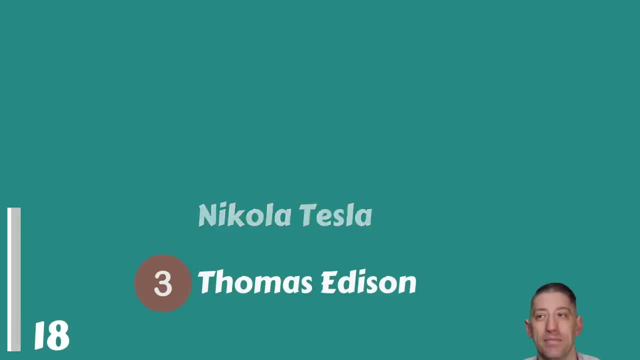 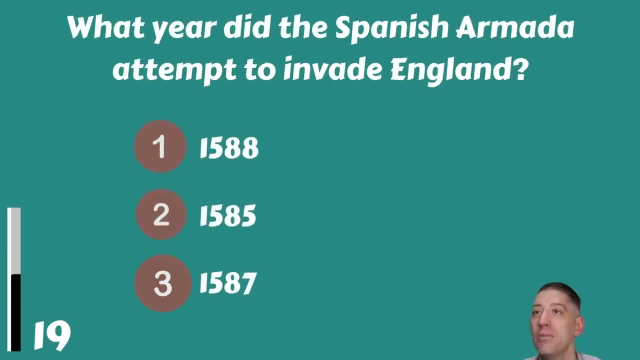 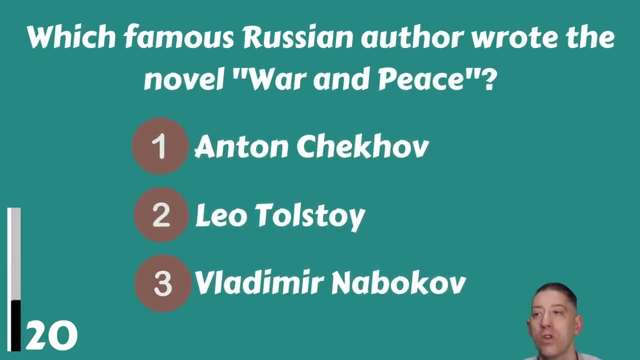 Nikola Tesla, Thomas Edison? What year did the Spanish Armada attempt to invade England? 1588,, 1585, or 1587? 1588. 1588.. Which famous Russian author wrote the novel War and Peace? Anton Chekhov, Leo Tolstoy or Vladimir Nabokov? 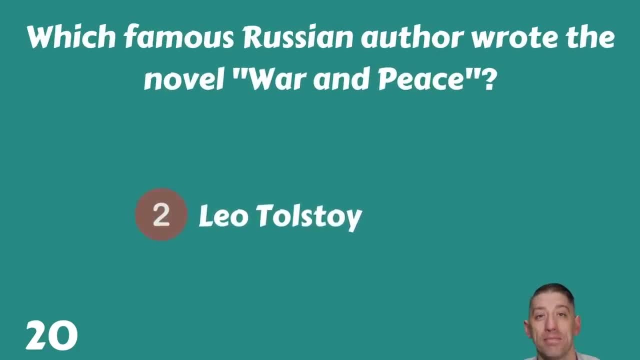 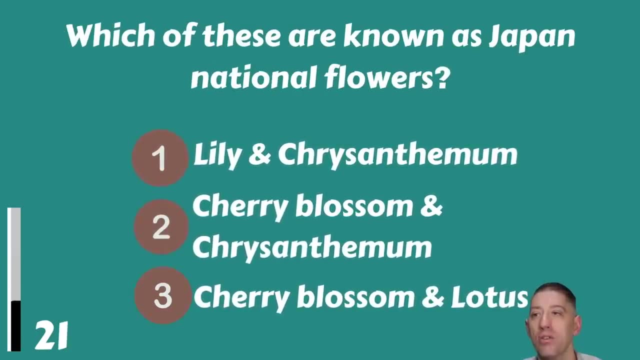 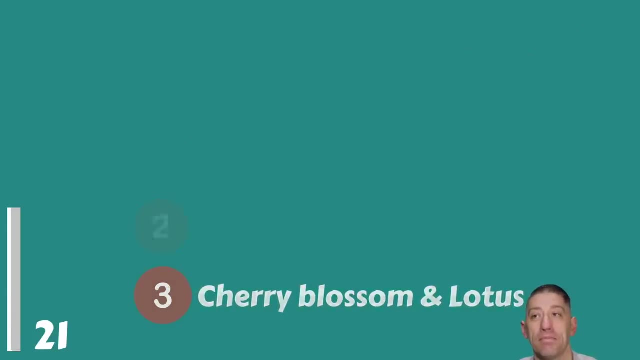 Leo Tolstoy, Which of these are known as Japan national flowers: The lily in chrysanthemum, the cherry blossom in chrysanthemum, or the cherry blossom in lotus, The cherry blossom in chrysanthemum. 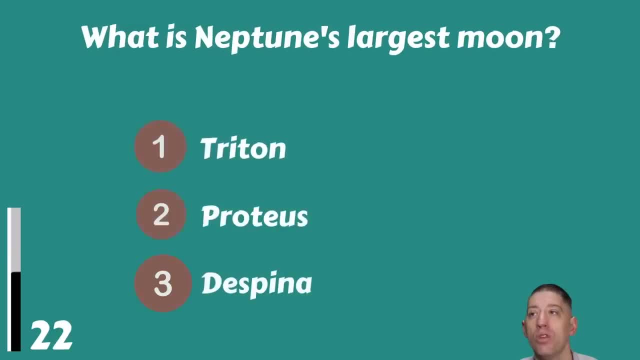 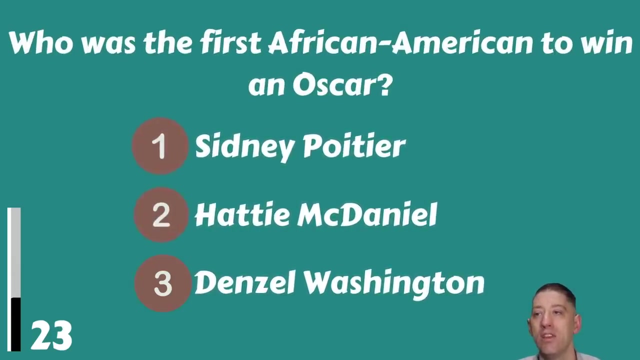 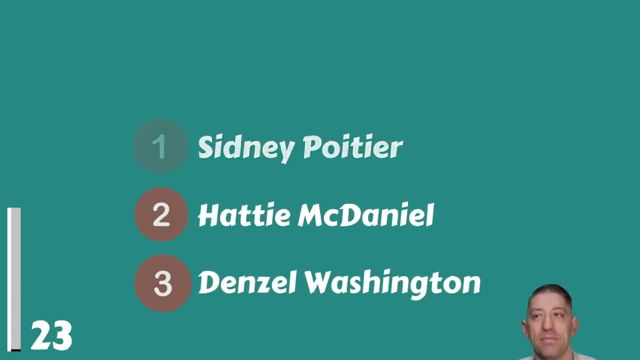 What is Neptune's largest moon? Triton, Proteus or Despina Triton? Who is the first African American to win an Oscar? Sidney Poitier, Hattie McDaniel or Denzel Washington, Hattie McDaniel? 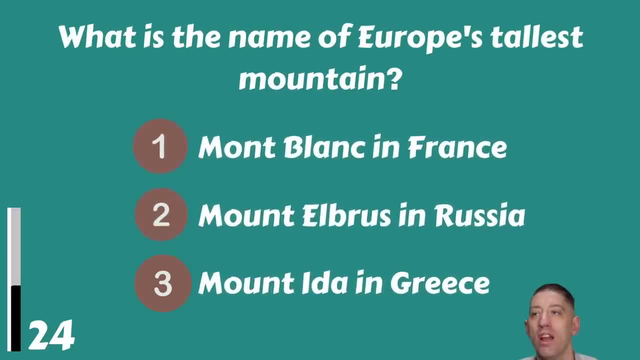 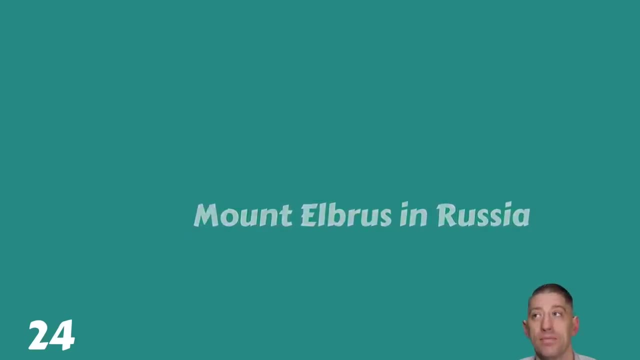 What is the name of Europe's tallest mountain? Mont Blanc in France, Mount Elbrus in Russia or Mount Ida in Greece, Mount Elbrus in Russia? What was the longest musical Broadway show of all time? Phantom of the Opera, Beauty and the Beast or Mamma Mia? 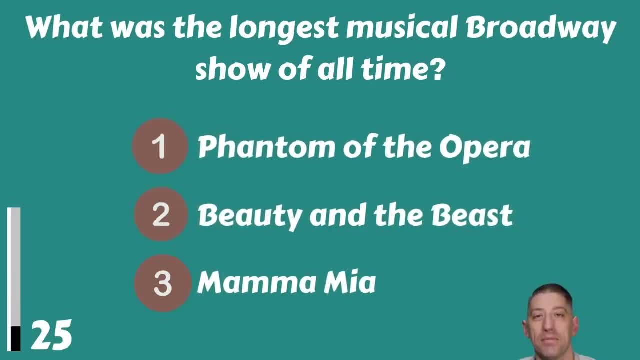 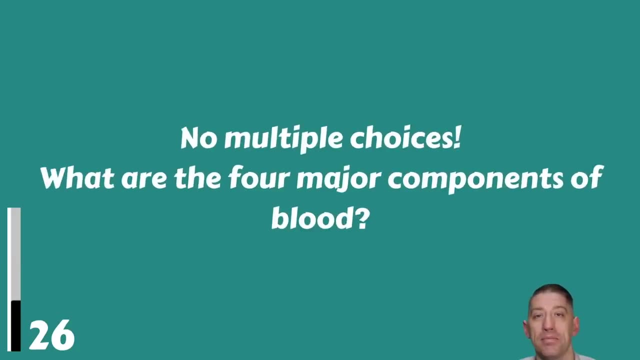 Mamma Mia, Phantom of the Opera. What are the four major components of blood? Plasma, red blood cells, white blood cells and platelets. What is a blood cell? A blood cell is a- photos 51.. A blood cell is a taką. 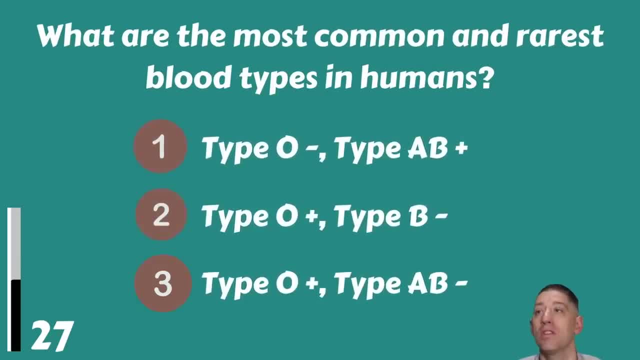 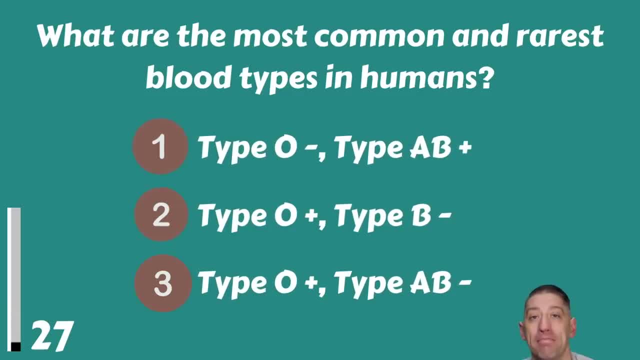 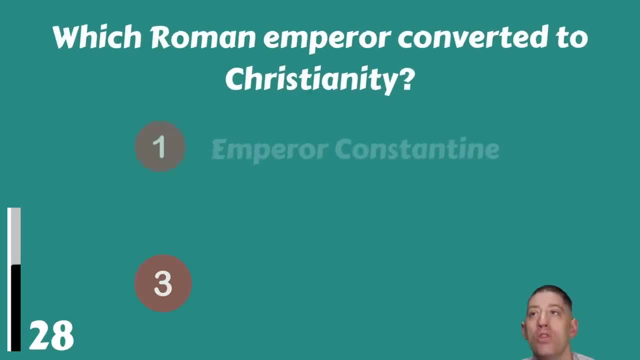 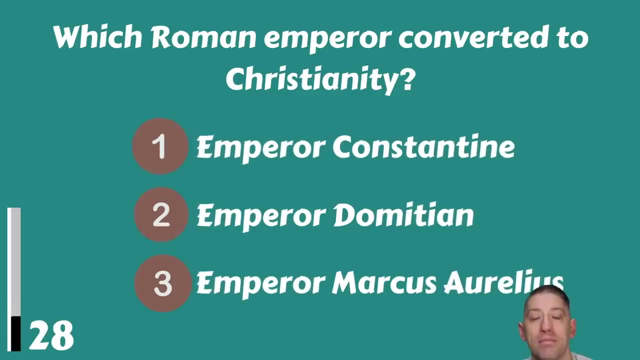 type O positive or AB negative? Type O positive and type AB negative. Which Roman emperor converted to Christianity? Emperor Constantine, Emperor Domitian and Emperor Marcus Aurelius. Emperor Constantine, True or false? Sydney is the capital of Australia. 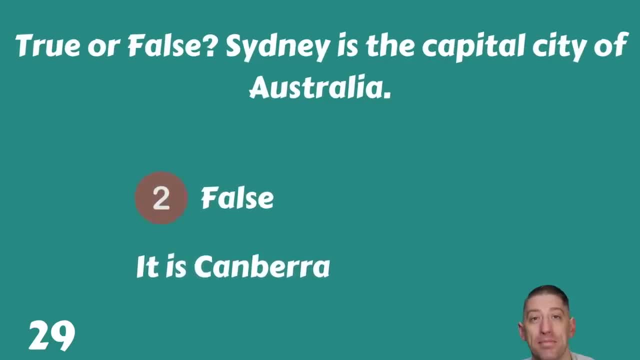 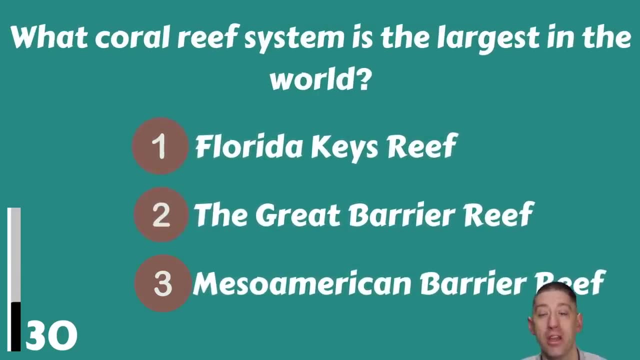 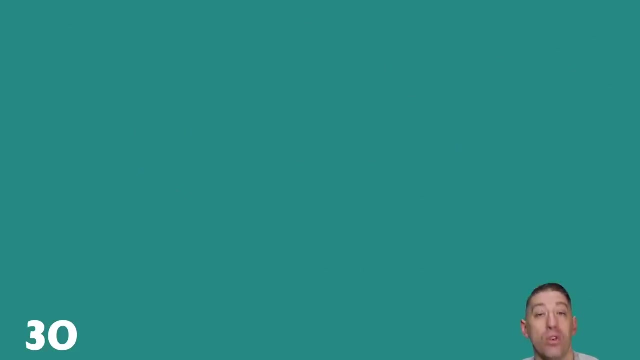 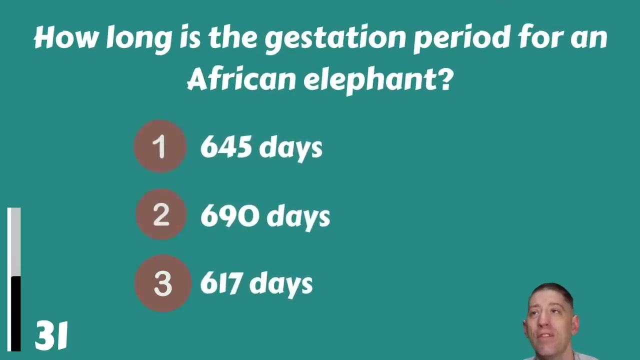 That's false. it's Canberra. What coral reef system is the largest in the world? Florida Keys Reef, the Great Barrier Reef or the Mesoamerican Barrier Reef? Florida Keys Reef, Floridaius- The Great Barrier Reef? How long is the gestation period for an African elephant? 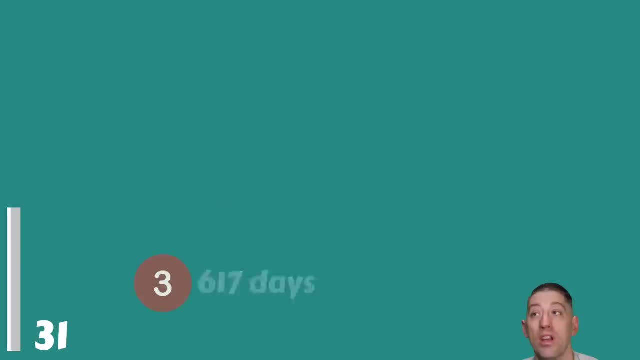 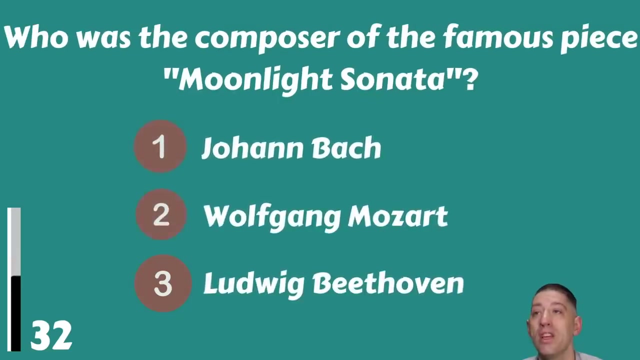 645 days, 690 days or 617 days, 645 days? Who is the composer of the famous piece Moonlight Sonata? Johann Bach, Wolfgang Mozart or Ludwig Beethoven? Ludwig Beethoven, What is a baby kangaroo called? 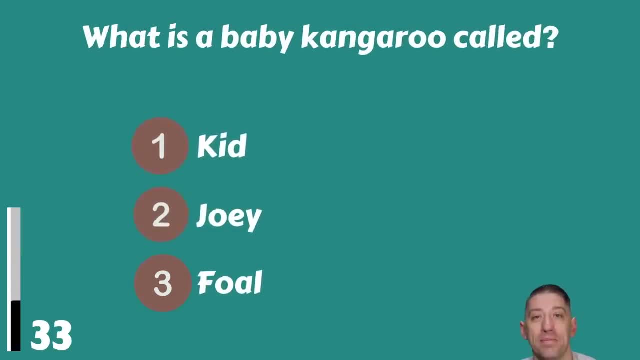 A kid a joey or a foal A joey? What year was the first Apple iPhone released? 2009,, 2008, or 2007? 2007.. What was the name of the first smartphone? 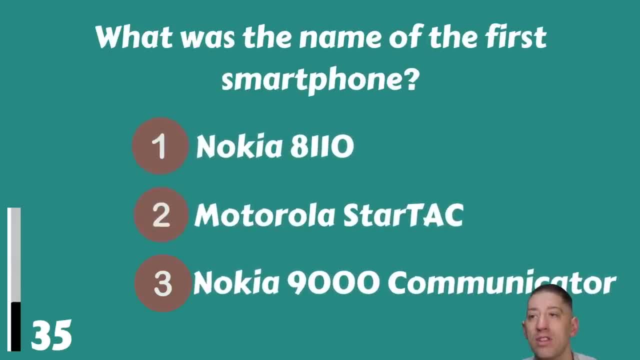 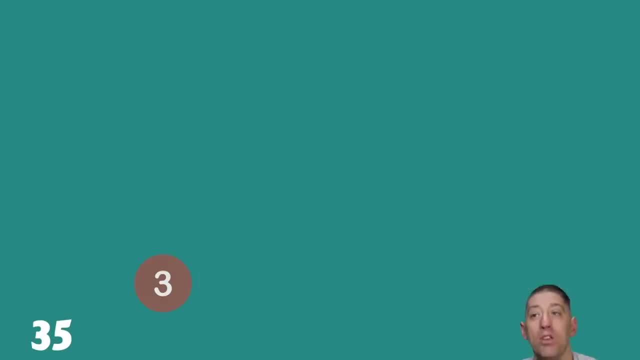 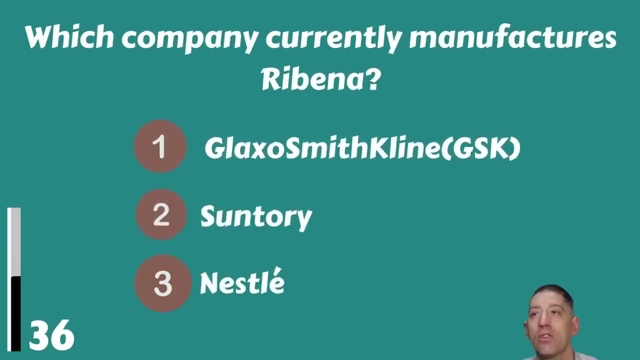 Nokia 8110? Nokia 8110.. Nokia 8110. The Motorola StarTAC or the Nokia 9000 Communicator? The Nokia 9000 Communicator: Which company currently manufactures Rubina, GlaxoSmithKline Suntory or Nestle? 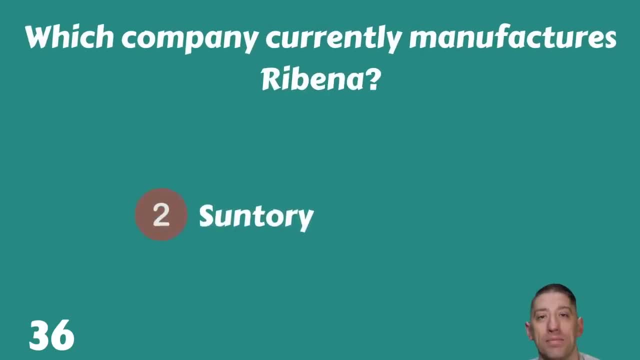 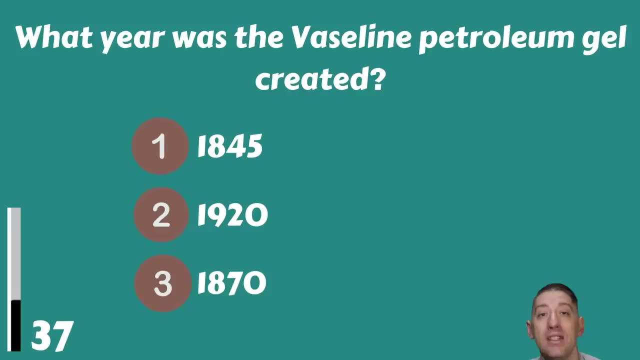 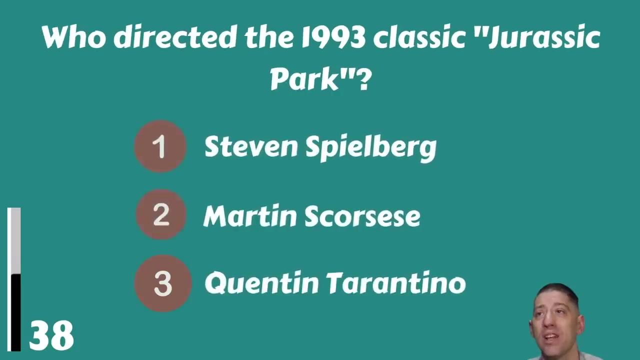 Suntory. What year was the Vaseline Petroleum Gel created? 1845,, 1920, or 1870?? 1870.. Who directed the 1993 classic Jurassic Park? Steven Spielberg, Martin Scorsese or Quentin Tarantino? 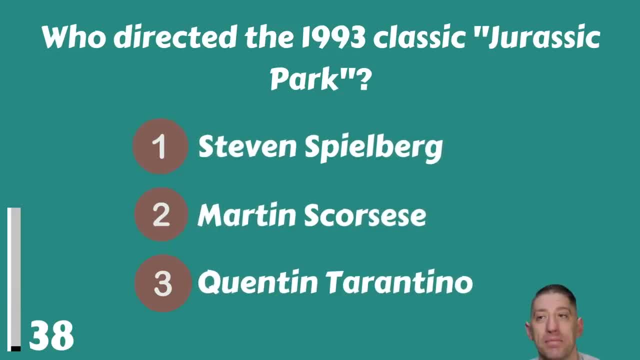 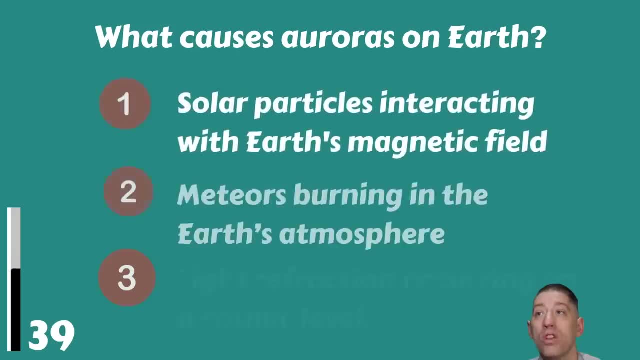 Quentin Tarantino, Steven Spielberg, Martin Scorsese or Stephen Spielberg, Steven Spielberg, Steven Spielberg, Steven Spielberg. What causes auroras on Earth? Solar particles interacting with Earth's magnetic field, meteors burning in the Earth's atmosphere. 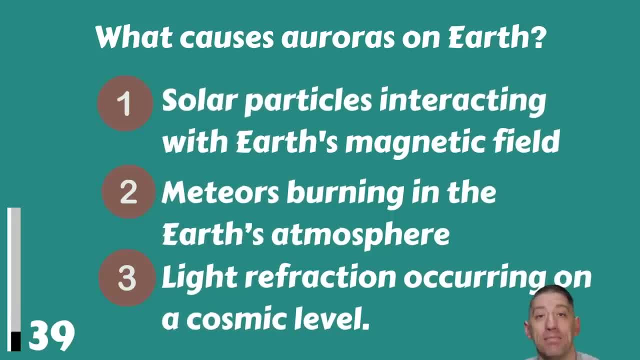 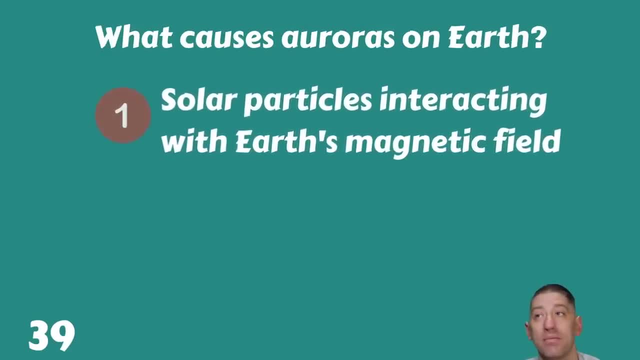 or light refraction occurring on a cosmic level, Or light refraction occurring on a cosmic level: Solar particles interacting with Earth's magnetic field. What is the sixth largest nuclear weapon? Who is credited with the discovery of penicillin? Norman Heatley, Louis Pasteur or Alexander Fleming? 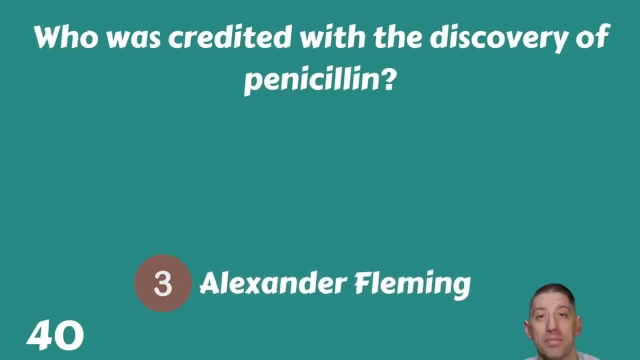 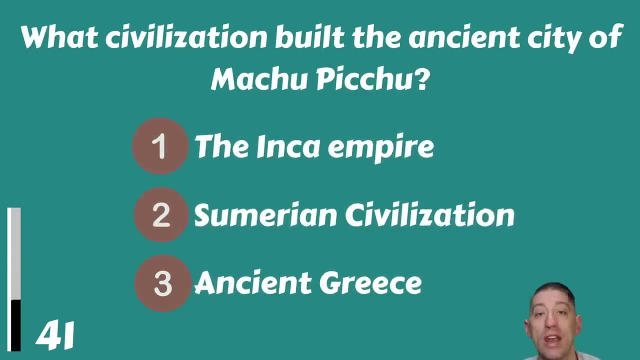 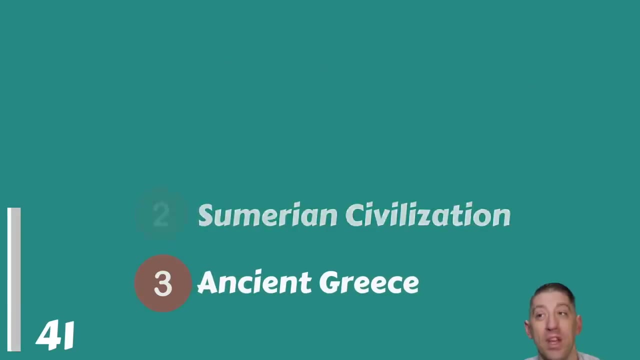 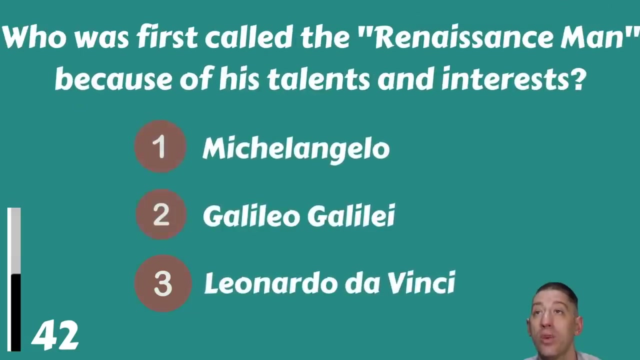 Alexander Fleming. What civilization built the ancient city of Machu Picchu? The Inca Empire? the Sumerian Civilization? or Ancient Greece, The Inca Empire? Who was first called the Renaissance Man because of his talents and interests? Michelangelo, Galileo Galilei or Leonardo da Vinci? 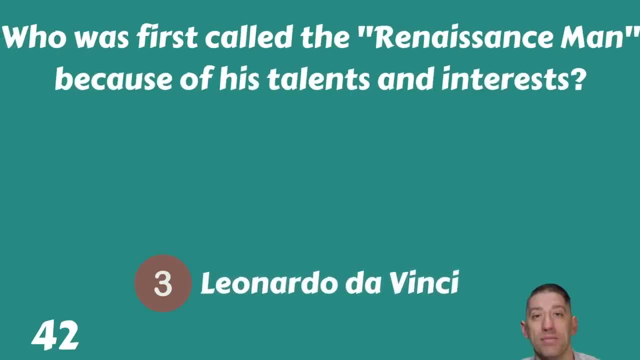 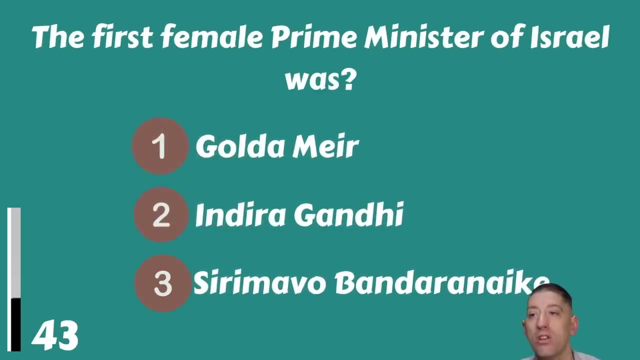 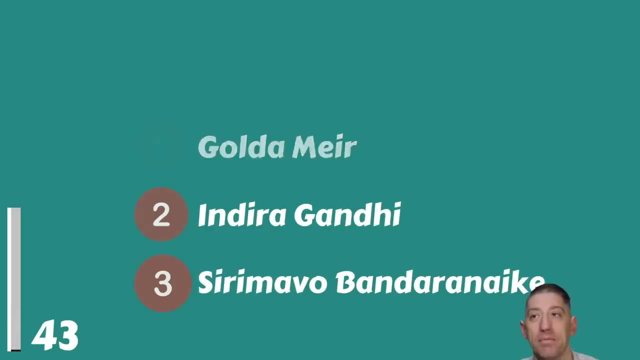 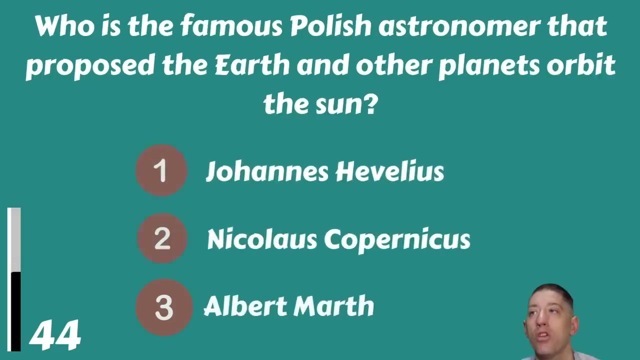 Leonardo da Vinci. The first female Prime Minister of Israel was Golda Meir. Indira Gandhi, or Sirimavo Bandaranaki. Golda Meir, Who was the famous Polish astronomer that proposed the Earth and other planets orbit the Sun. 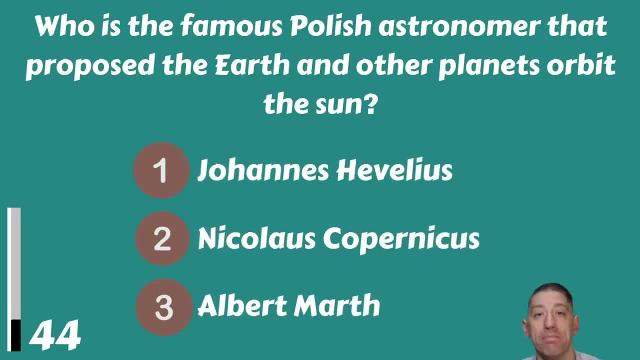 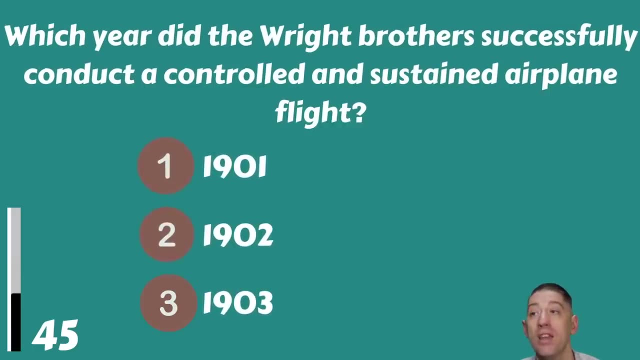 Johannes Hevelius Nicolaus Copernicus or Albert Marth Nicolaus Copernicus? Which year did the Wright brothers successfully conduct a controlled and sustained airplane flight? 1901? 1902, or 1903? 1903.